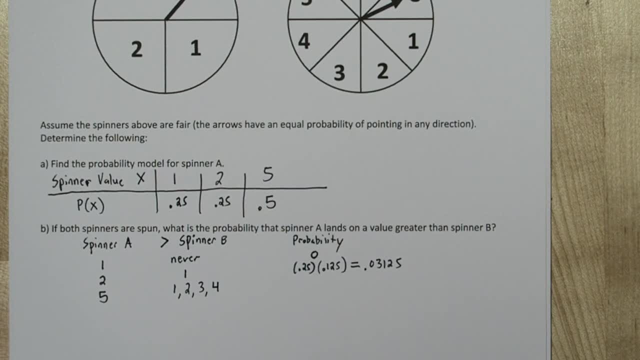 3, and 4.. Let's start by figuring out the probability that spinner A lands on 5, and spinner B lands on 1.. Since they're independent, we can multiply the probability spinner A lands on 5,- 0.5, by the probability that spinner B lands on 1, 0.125.. 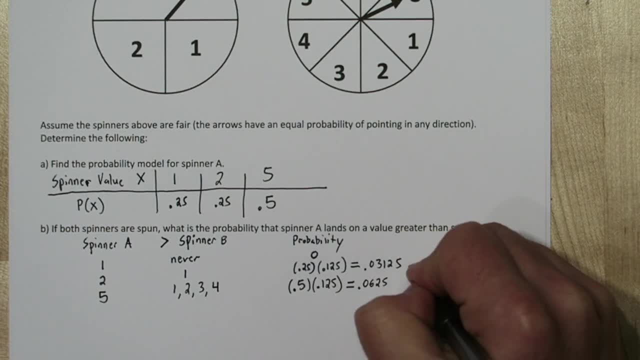 So this is our probability of getting a 5, 1.. A 5 for spinner A and a 1 for spinner B. Now, since the probability of getting a 5 for spinner A and a 1 for spinner B is: 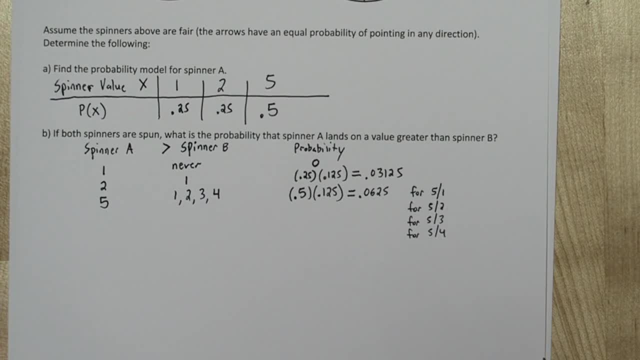 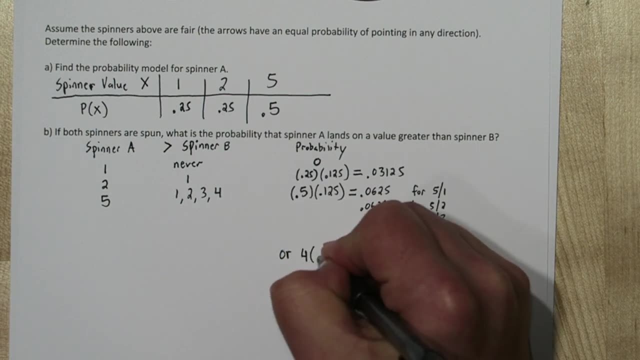 the same as getting a 5 for spinner A and a 2,, 3, or 4 for spinner B. we can just copy the probability we got for the 5, 1 scenario, Or we can just multiply it by 4.. 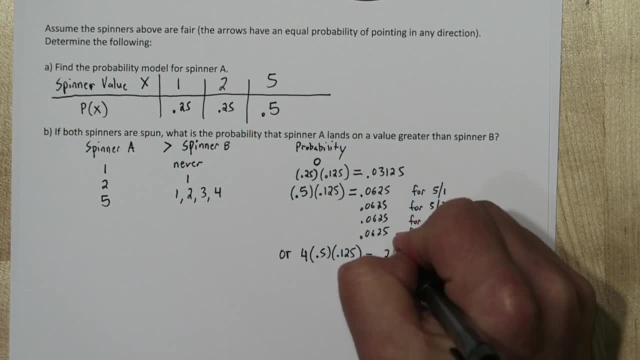 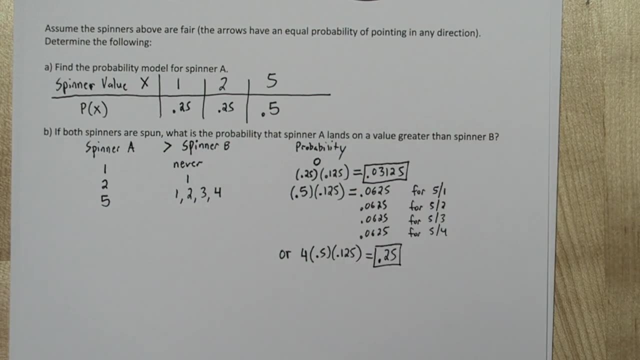 It turns out, the probability of getting a 5 on spinner A and then a 1,, 2,, 3, or 4 on spinner B is 0.25.. So we're left with three probabilities. Our zero probability is the probability spinner A lands on a 1, and is greater than spinner B. 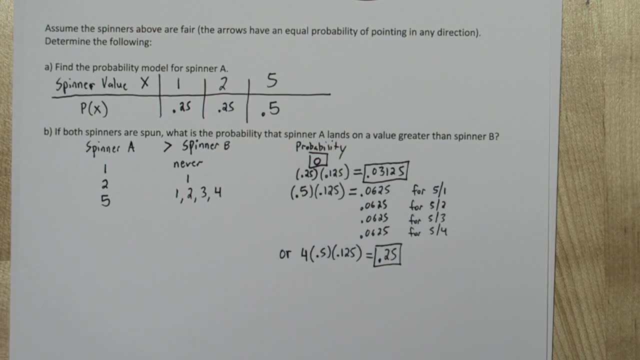 Our zero, three, one, two, five probability is the probability spinner A lands on a 2, and is greater than spinner B, which happens if spinner B lands on a 1.. And finally, our point-two-five probability is the probability spinner A lands on a 5,. 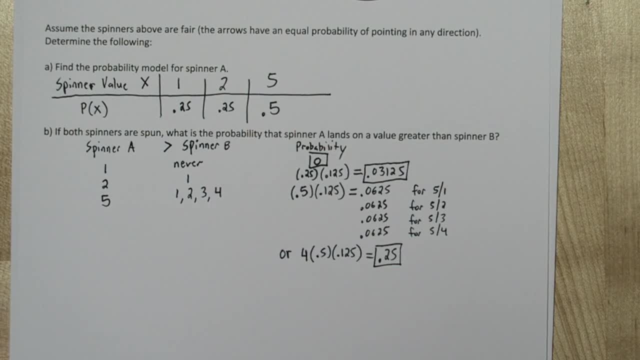 and is greater than spinner B, which happens if spinner B lands on a, 1,, 2,, 3, or 4.. So if we add these three probabilities up, we have our total probability that spinner A lands on a value greater than spinner B. 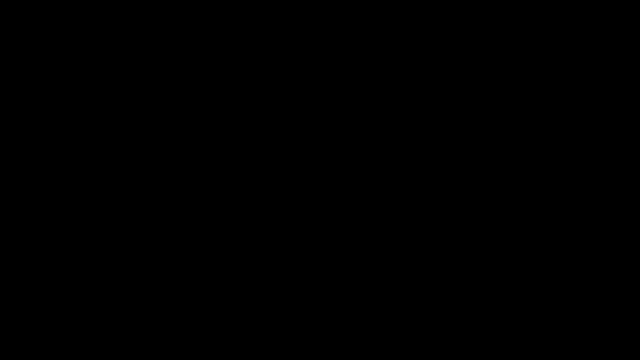 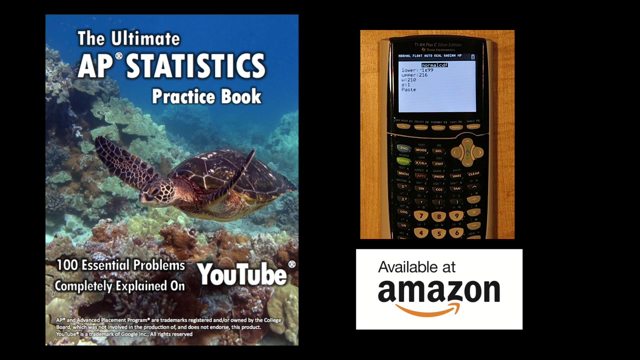 B Like this video. Check out my book, The Ultimate AP Statistics Practice Book. It's got a hundred problems, all with videos just like this. You can pick it up on Amazoncom.